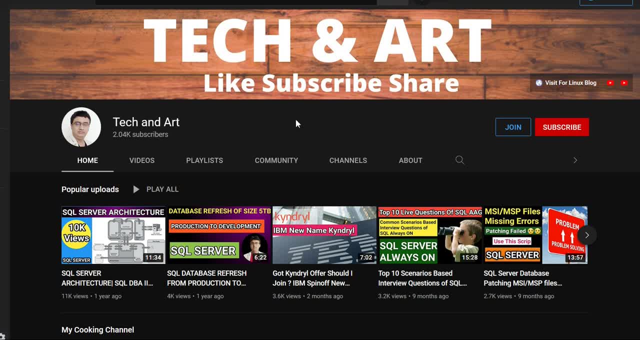 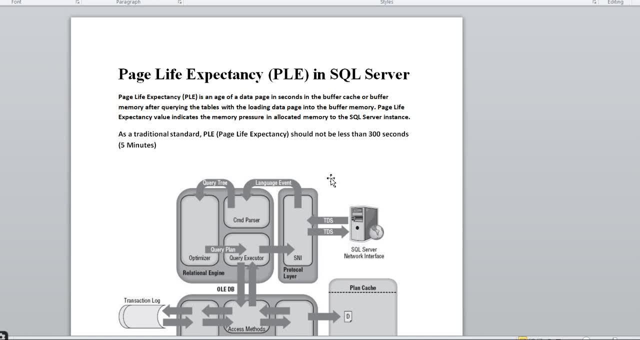 So let me start the today's session actually. So we have. we will go with the couple of scenarios I have created. the one nice documents about to better understanding about the PLE, the page life expectancy in a SQL server. So basically the page life expectancy is an age of data page in a second in the buffer cache or buffer memory. after querying the tables with the loading data page into the buffer memory Page, like life expectancy values indicates the 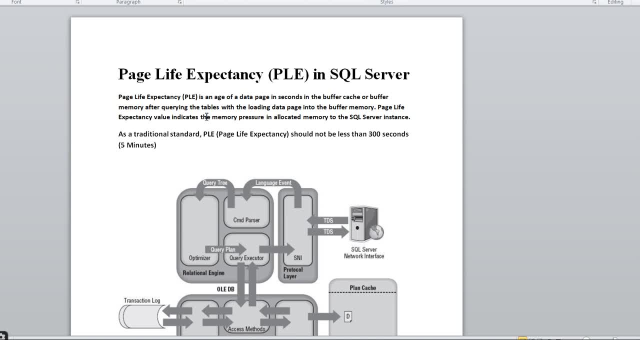 memory memory pressure in allocated memory to sql server instance. okay, so basically it's saying the your page life expectancy database how much seconds waiting in your buffer memory. okay, so by default it's a setting. is a traditional standard ple counter is not less than 300. 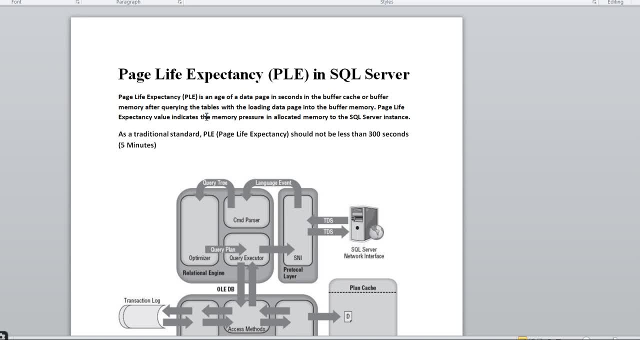 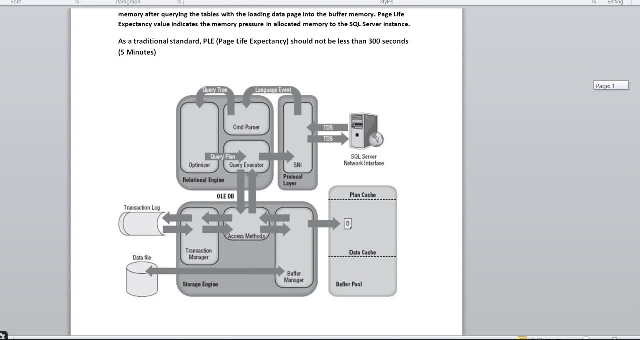 seconds, which means the five minutes. okay, so we'll understand this clearly in a better way in this with this help of this diagram. I have already covered this diagram in architectural video. okay, how the query is processing and what is the ple. so we can understand the ple. 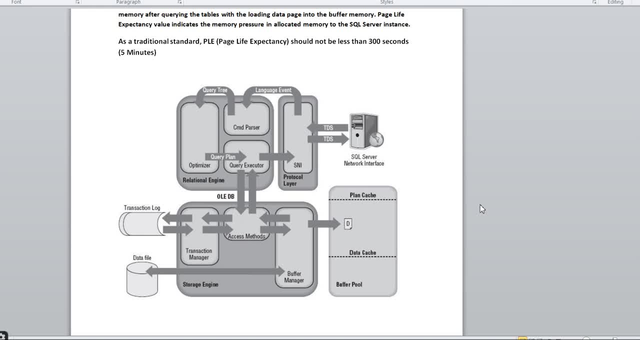 in this with the help of this diagram. so if you have visited my, you know if you watched my sql server architectural video, so you have the better overview about this, so you can understand this diagram. so sql server engine is divided into two parts: relation engine and storage engine. so whenever we are hitting the query, so it's like firstly it's coming. 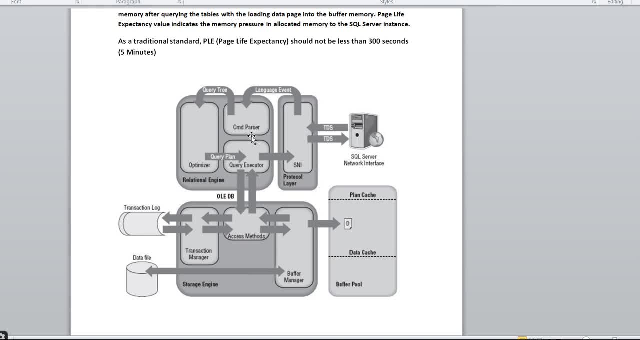 the relation engine to from the protocol layers to command parser and the optimizer and the query executor. and query executor will send in the query to the storage engine access method. in access method you know it's going to check the select or non-select query, so I have already covered. I'm not going to discuss in details how the query is processing in. 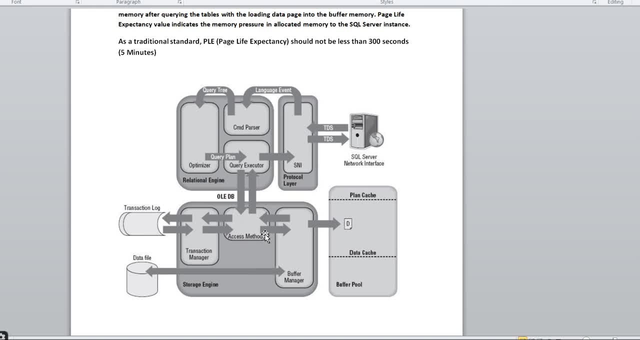 a second sql server engine. you can watch my architectural video, okay, but here in a buffer memory, a couple of things as we already discussed in architectural video also, but in in this session I'm going to tell you, in a buffer model we have a database. okay, this page, this is called database. so 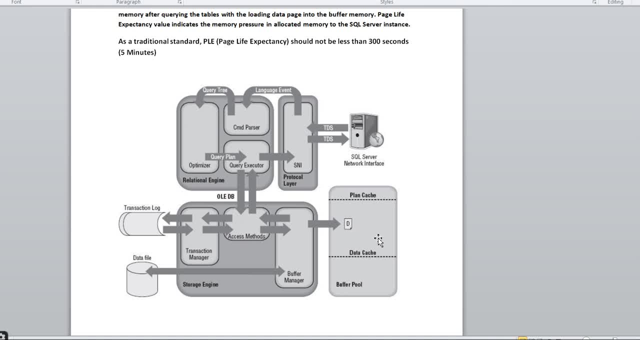 here is the classical role of ple, so, which means how many seconds your you know data is available in your buffer memory, okay, so the default size is. default time period is 300 seconds, which means 5 minutes. okay, if it is less than 5 minutes, then there is a really really memory chunk, okay, so if you take 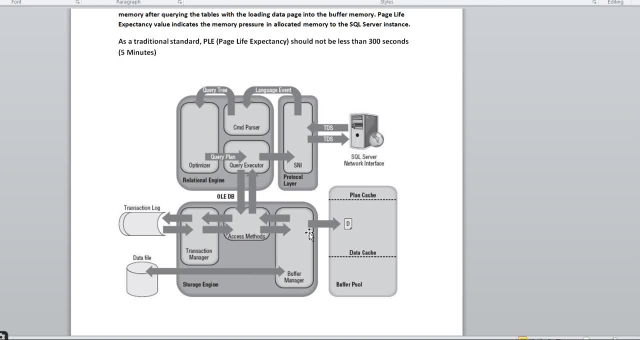 the example, if any query is come your, you know coming through this way and you know if the data is placed in a data Buffer, memory, data cache, if you know the data case size is not huge because we all aware, you know, or these dataー this data is flush out after the sum period in term of interval. okay, so this data is not. 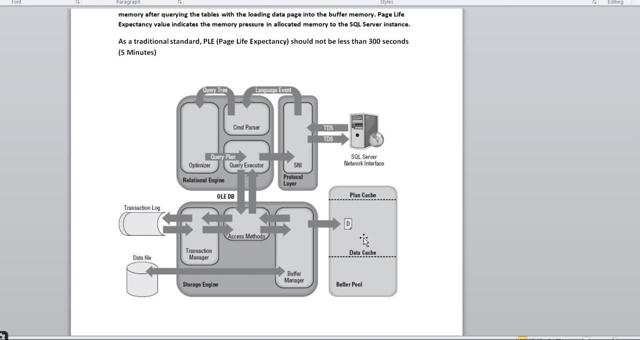 presently for longer time. after the sum interval, it's going to flush out. so there is another process called, you know, log writer- writing data from the database to database files, and they are doing the flush out based on the scenario. okay, so forget about that. so the the thing is here. 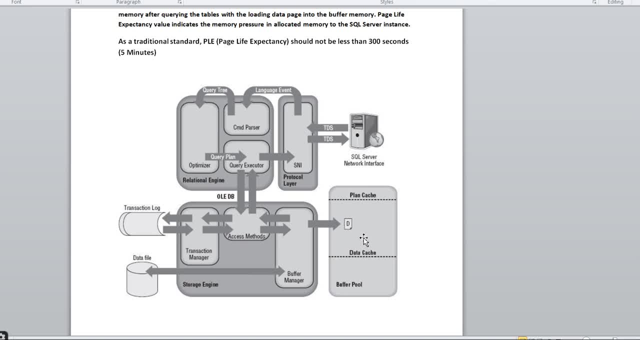 how many seconds your data is available in your buffer memory. okay, this is called the PLE page: life expectancy. that should not be less than 300 seconds, which means the five minutes. if you take the example, or you have a- you know- capacity of 10 people, you have a 10 chair. 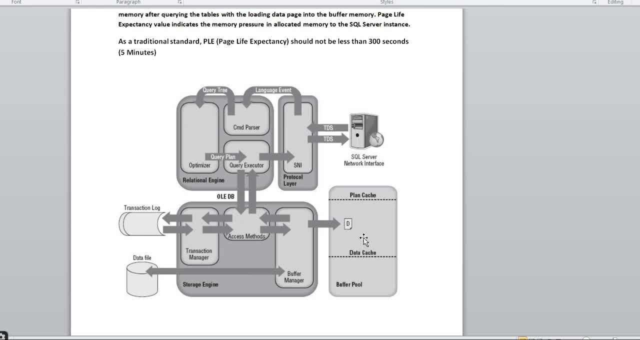 something like that. so suddenly, 5 more people came. so now you have only option is: you know, you need to, you need to, you need to are in a pressure, you need to release the older person- old, old people who have already captured the chairs- and you can, you know, give the chance to further new resource, or either you need to. 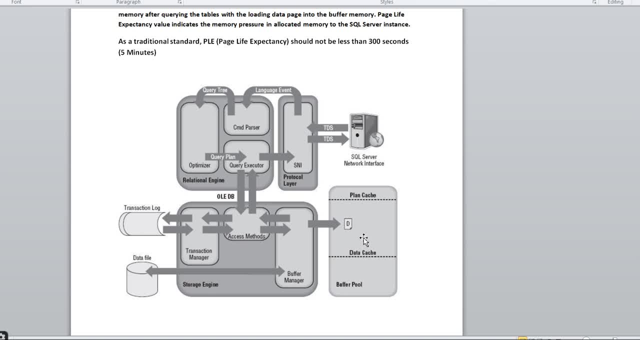 increase the size from 10 to 15, right. if you have a capacity to increase the size, then it's okay. if you don't have the size, so- which means you are in a pressure now, either you need to release the people, whoever already captured that chair, and you can give the chance to the new, newer people. 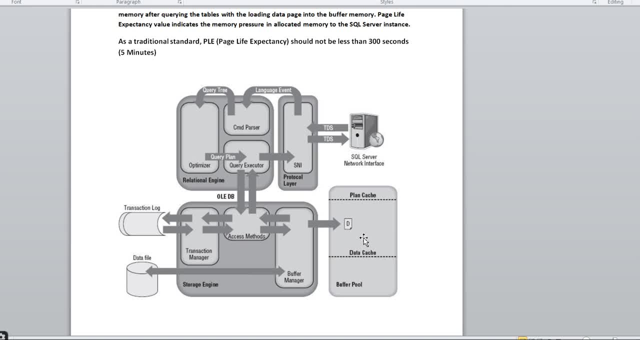 and either you can increase the size. so same thing here also: if data used in your buffer memory, the data cache size, is not huge, not big according to your server memory setting, then there will be a process, there will be a pressure in a memory. okay, if size is, you know, big, then you can, you know. 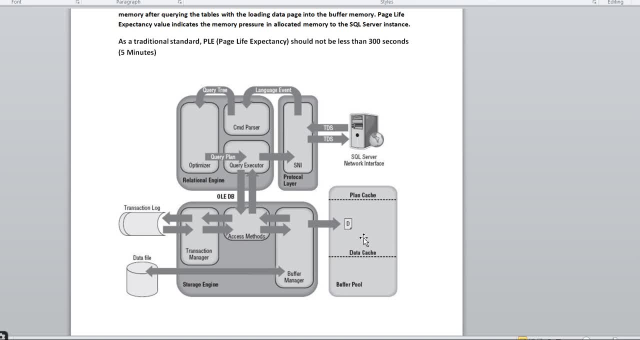 give the chance to the new process, or otherwise you need to flush out the older data from your buffer pool. okay, so this is the process, so that flustered process, if, if it is not holding five minutes, you know something like that, your, uh, you know transaction is too high and it's like you know, buffer memory is not holding. 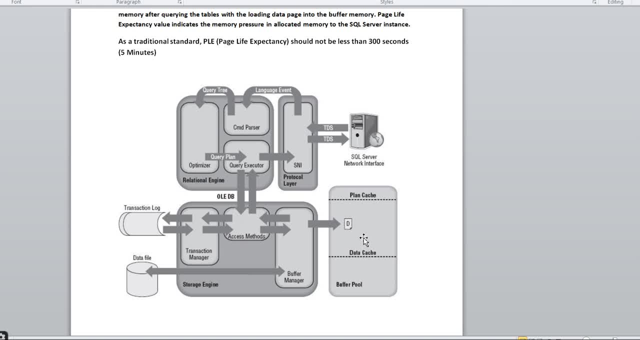 any transaction in buffer, buffer memory in a database. uh, five minutes as well, it's, it's like below five minutes, then there is a memory pressure in your service equals our instance. so this is the agenda here. uh, for ple actually. so now the point is how to calculate the ple. so we'll. 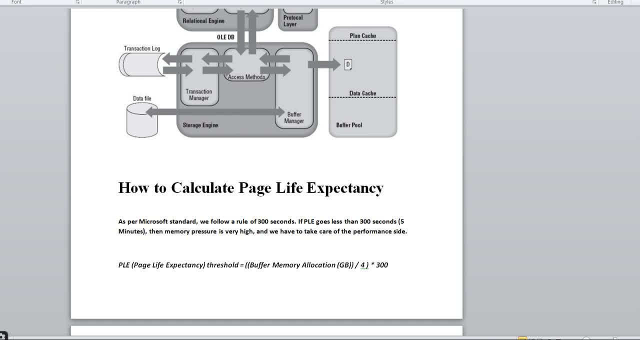 understand this way. see, the default size is 300 second. that is the default counter, which means five minutes. but based on your sql server instance memory, you need to calculate. you know what should be the exact counter. okay, so we can understand with this calculation what will be the perfect. 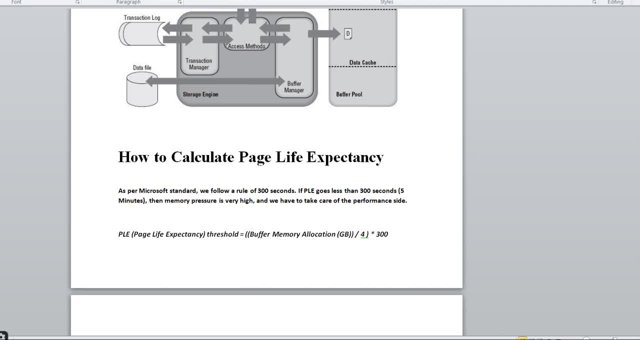 ple counter for my instance. okay, the 300 second is a default instance, a default counter from the microsoft. but what is the my instance, how much server memory in my instance and what should be the ple counter? so we can understand with this, you know, uh, calculation. so, as per the microsoft standard, we follow the rule 300 seconds if ple goes less than 300 seconds. 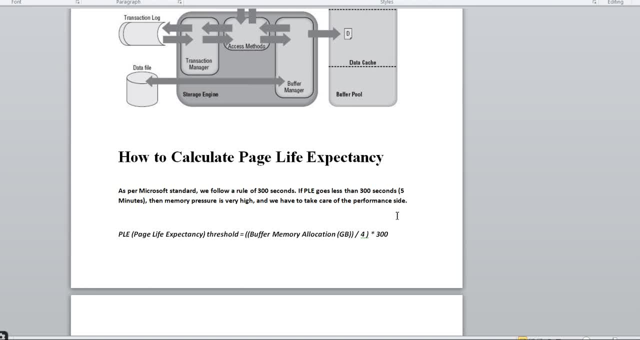 then the memory pressure is very high and we have to take care about the performance set. as i said, microsoft recommended 300 seconds only. if less than 300 seconds, then there is a problem. so this is the default. now the point is how to calculate. so this formula will give you the exact. 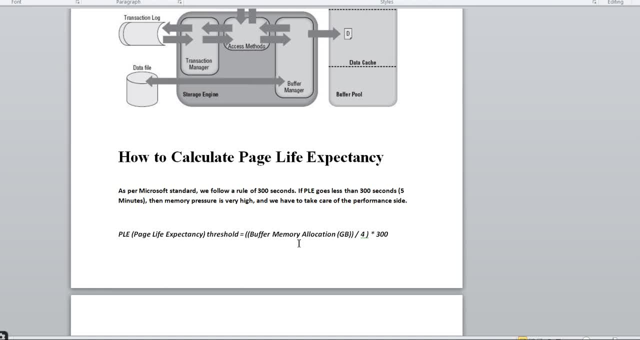 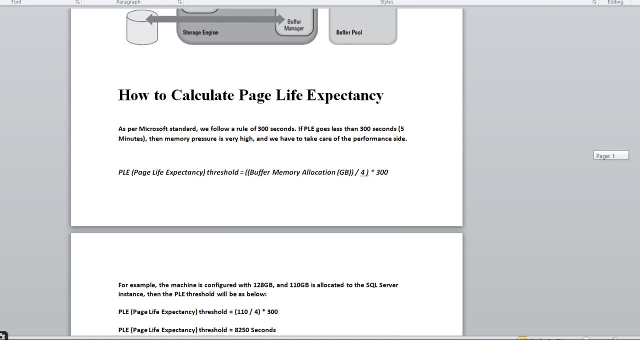 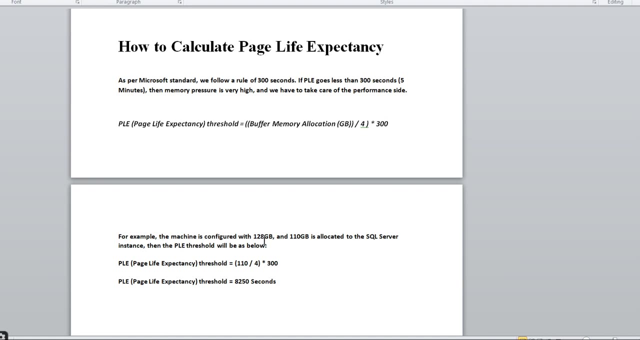 overview: ple threshold equal to buffer memory allocation in gb by 4, multiply by 300. so this is the formula. so if we can take an example for this formula, so if you can see here, for, for example, the machine is configured with 128 gb and 110 gb is allocated for the sql server, so total server memory is: 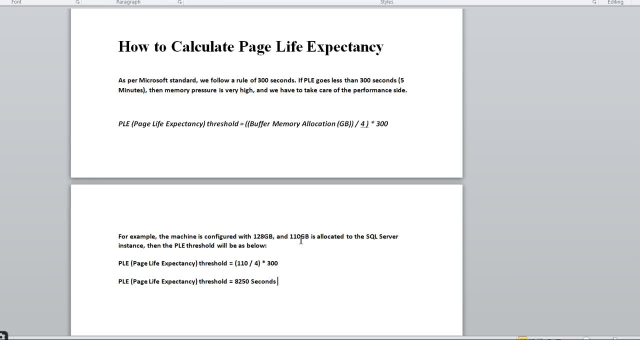 and 110 gb we are giving for the sql server instance. so in this case, what should be the exact ple counter so we can place this value in this above formula? ple is equal threshold equal to 110, what we have allocated for sql server instance divided by 4, multiply by 300, so it's 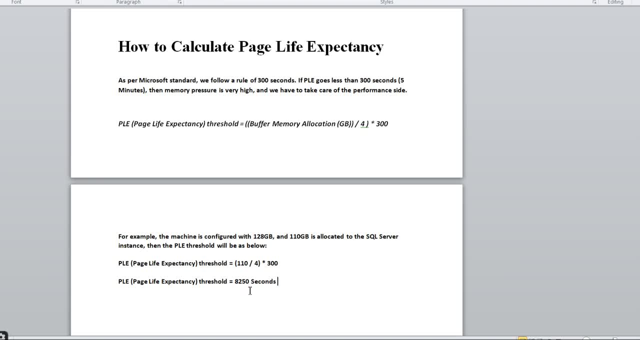 coming like 8 to 5: 0 seconds. so your ple for this instance is 8 to 5: 0. okay. below 8 to 5: 0, then there is a memory pressure you need to figure out. either you need to increase the memory or you need to see why this memory crunch is happening. need to do the troubleshoot. 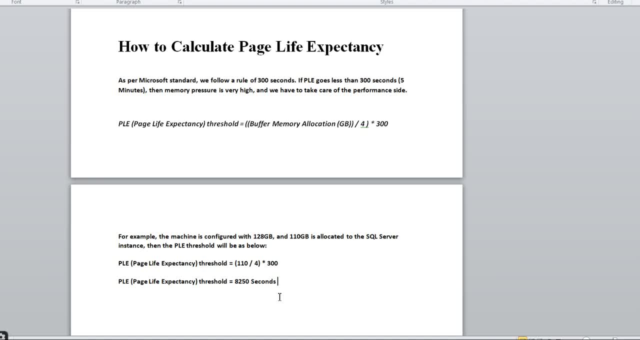 but the finding, the exact calculation for ple. this formula is really really helping. okay, the default is 300, don't believe. if more than 300, uh, you can assume my instance is, you know. okay, it's not in under pressure, you need to figure out for your instance, boss, you can. 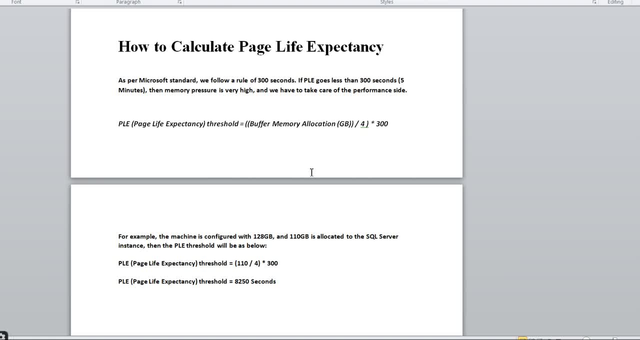 place this uh value: uh, you can place this value for on this formula to get the exact ple counter. now i will show you the query: how to uh find the exact ple counter. okay, for the sql server instance. okay, how to check. so let me connect my name: studio. if you can see here, we can use this. 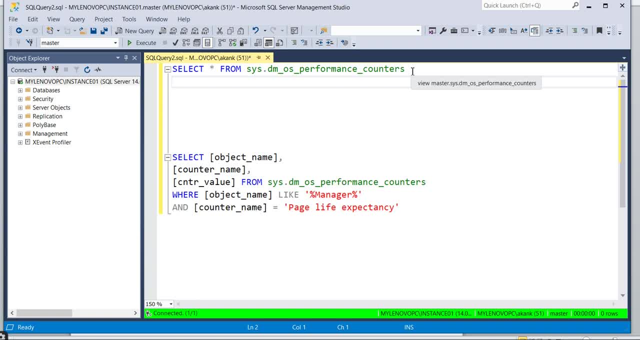 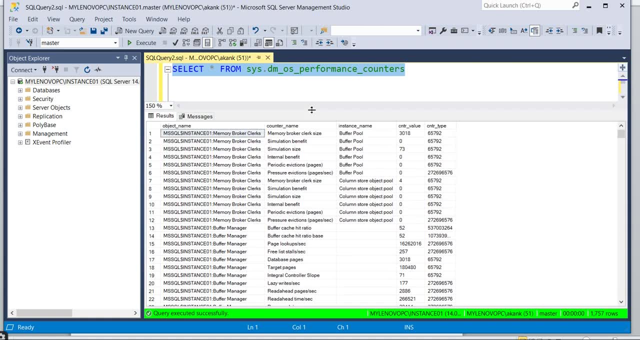 sys objects command sysdmos- performance counter. this counter will give you the lot of things actually if you execute. if you can see here lot of counter is you know you, which can help you to analyze the uh, performance tuning actually. so one of the counter is ple buffer. 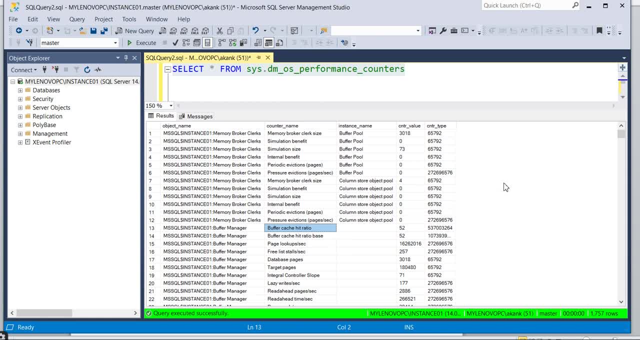 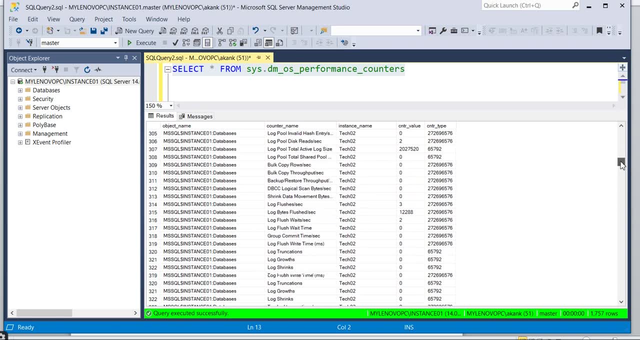 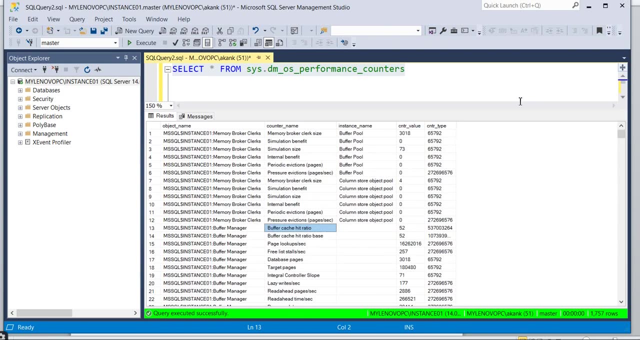 buffer catch hit ratio also. you can find it from this command. so lot of counter is there. counter value is there. you can utilize this sysdmos performance counters which give you the exact, you know- details about your sql server instance and data base. okay now, uh, in this session i am going to discuss about only the ple. so what i have? 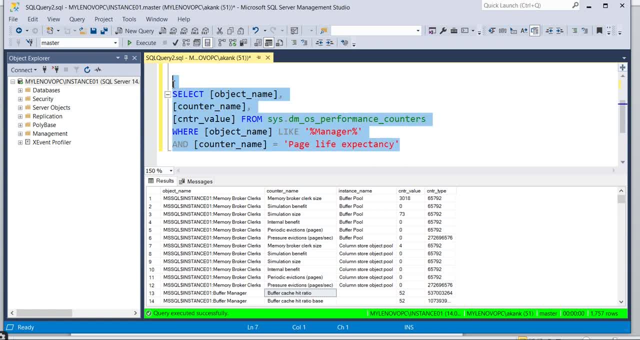 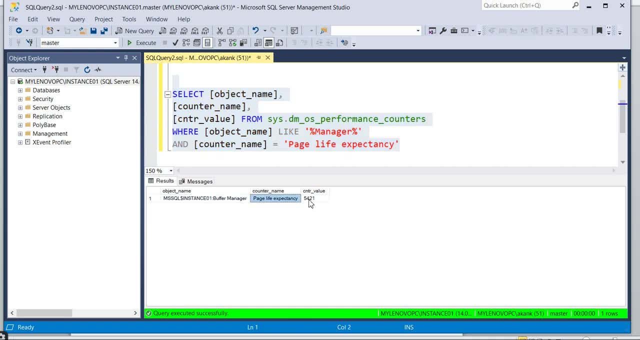 did it actually? i have placed the you know filter here and i'm going to execute. if you can see here now i am getting only for the page life expectancy. so my counter value is 5, 4, 2, 1, so which is really okay with my sick lab sql instance, okay. so in your case, what i have did, uh, discussed here in this, 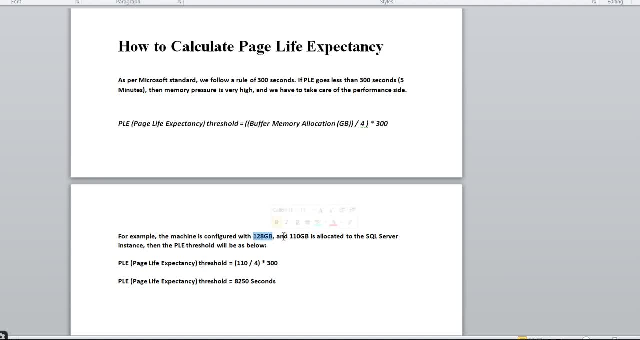 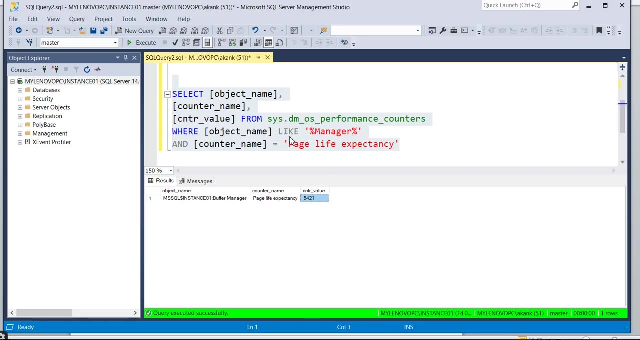 session is that you have to figure out what is the server total memory and what you have allocated for sql server. then place this value in in this formula and what the output will come. that much seconds is your ple for that particular instance. okay, so you can use this script to identify what. 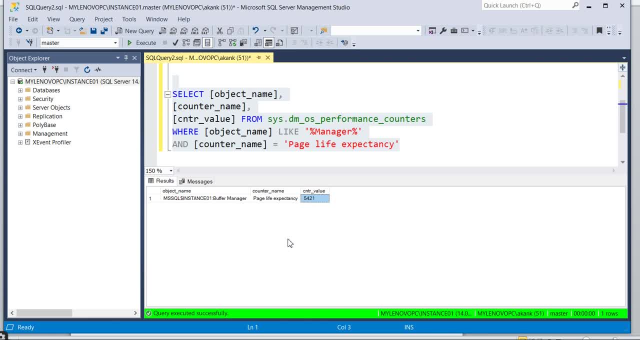 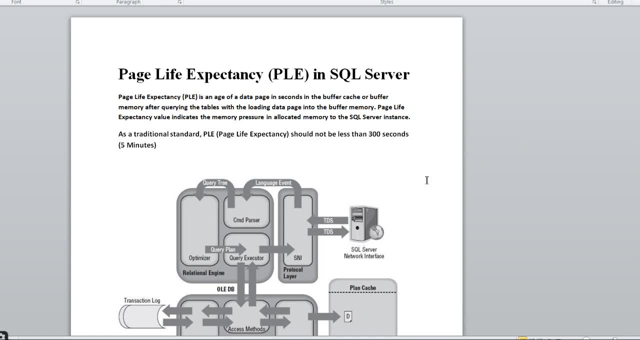 is the ple counter for this instance? okay, i will give this script in a description and hope you got my point what i try to say. this in detail session: what is the ple and when it's coming? uh, sql server memory pressure, what should be the exact threshold for your particular instance? how to figure out what is the current? 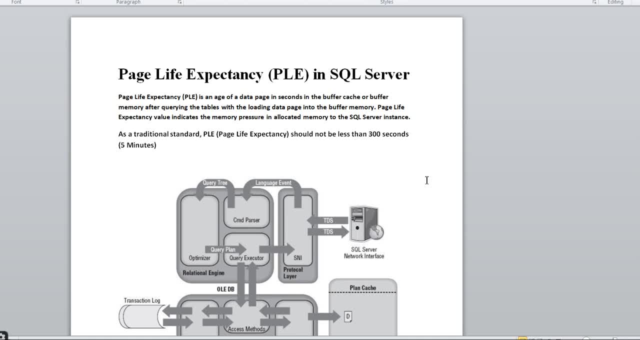 ple with the help of this script and what should be that actually you can calculate based on that formula. okay, hope you got the point. what is the ple? just a one line statement you can say in an interview. also a lot of questions come. what is the page like? so ple is nothing, just how much second your uh buffer memory is holding for database. okay, 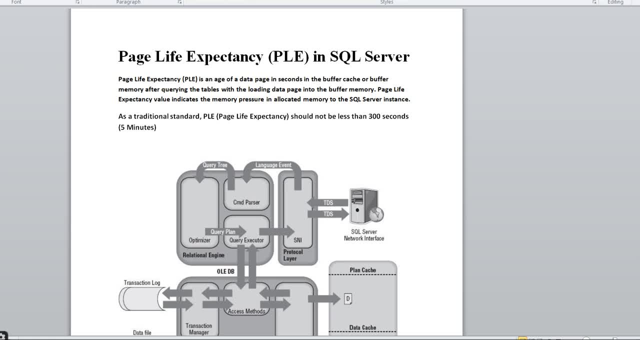 if less than so they will ask: what is the counter? so counter is 300 seconds. but you know it's a default counter but it's not for your sql server instance. so for your instance you need to calculate. suddenly they will ask how you can calculate for the. you know for your own instance. 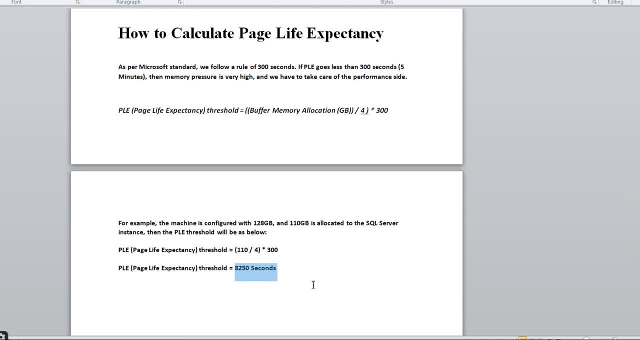 they will give the scenario also like this. only so i have seen in a number of interviews they will put the some scenario server memory: is this much sql server? you have allocated this one how you can calculate the ple. so you can calculate the ple based on this formula. actually they are. 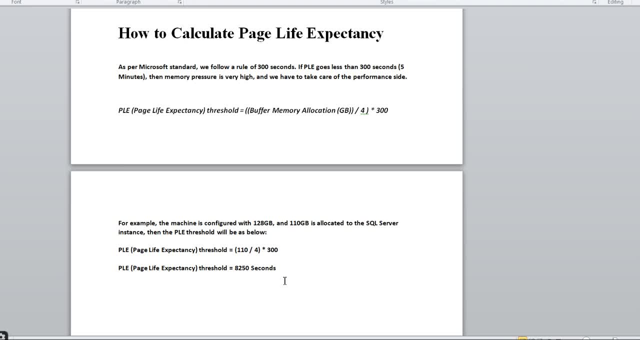 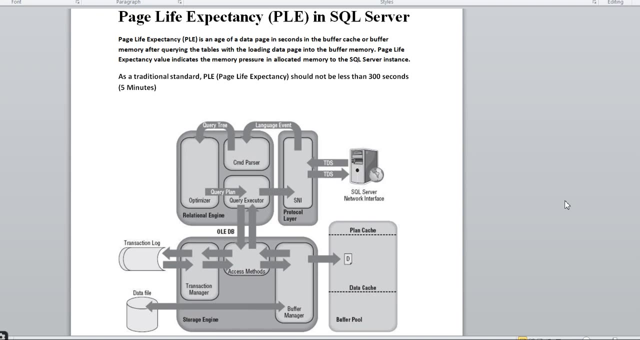 just looking for this: whether you have a knowledge or or not, how to calculate the ple for a particular sql instance. so this video i think i have provided a lot of information. we've covered a lot of interview questions also and for better understanding. uh, you know, you can do the testing on your sql instance. 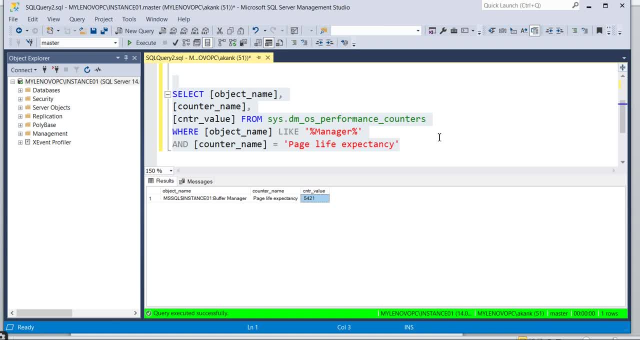 execute this command to find out the exact ple counter and if it is not, then you you can also calculate your server memory based on the server memory and allocated sql server instance memory and you can put the you know, then you can, you can figure out what should be the ple actually. 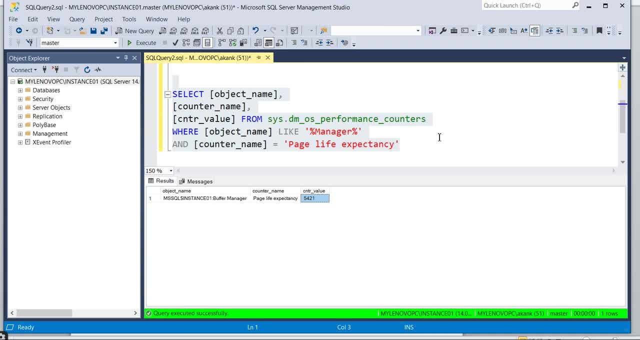 hope you got the points very soon. i will meet till then, bye, bye, thank you.